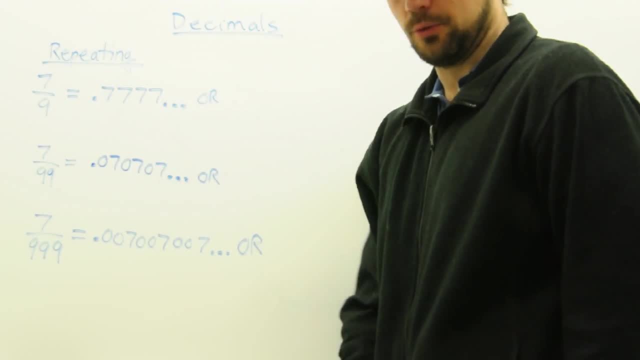 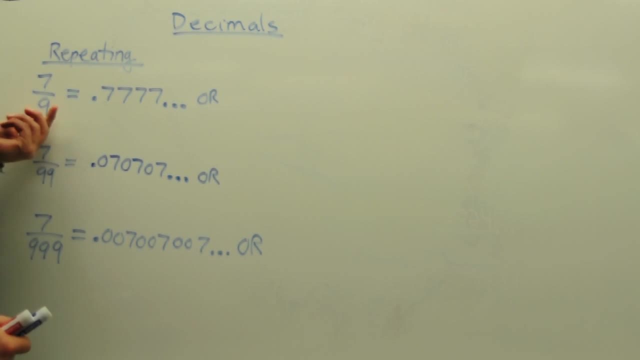 That's a guarantee. if you were to actually do the long division and figure out what that would be, We can recognize there's kind of families of repeating decimals. Here we have 9s, 99s and 999.. Let's think of it this way. 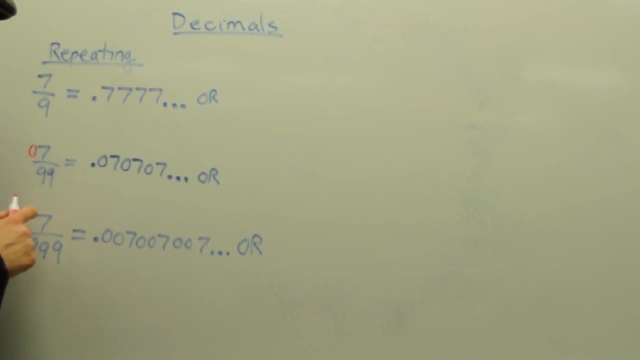 This is the same as 0, 7.. Two digits, two digits. How about three digits here: 0, 0, 7.. It's very easy to tell what our decimal is going to be: Three digits, three digits. 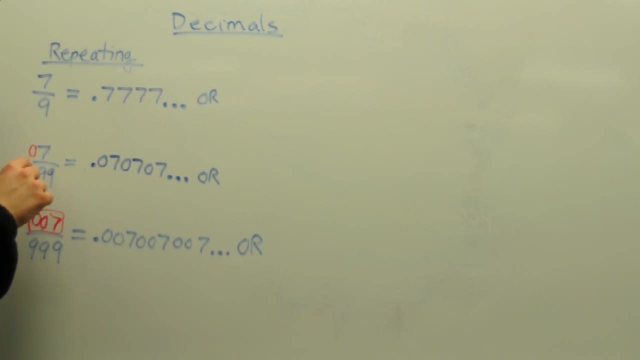 Okay, well, it's the three digits are what repeat Here. if it's two digits, it's two digits that are going to repeat Here. it's one digit, one digit, It's the single digits that's going to repeat. 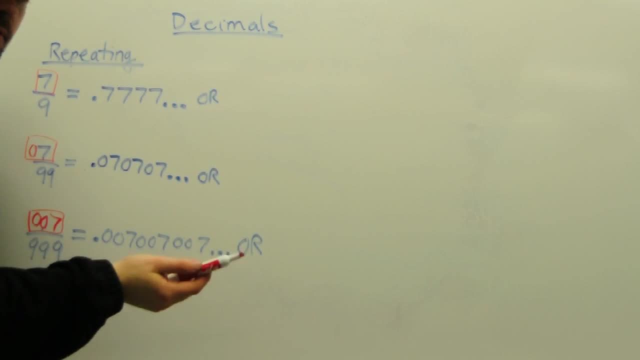 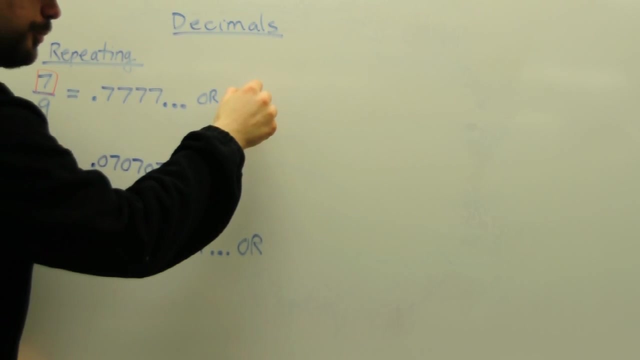 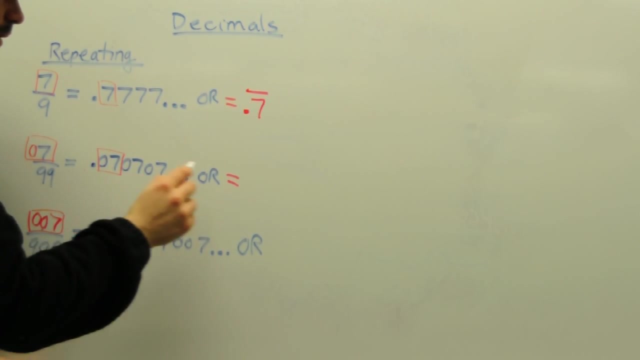 Now just to note about notation 0.777, whatever. we know that that is going to be able to be written like this: 0.7, with a bar over top of it. okay, That is what repeats. Now this one, it's the 0, 7 that repeats, so we know that our answer is 0.07.. 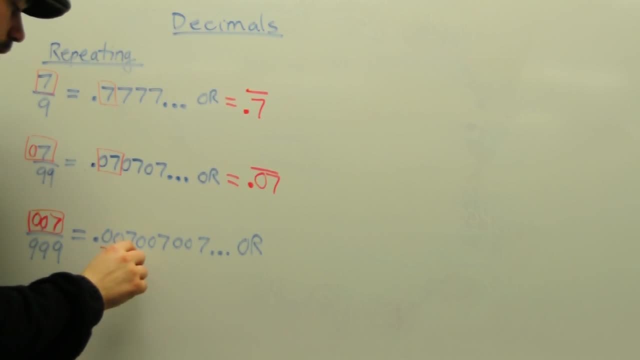 The bar goes over top of the 0 and the 7. And this one, the part that repeats, is 007, so our answer here is 0.007, and the bar repeats. What's important here is this pattern: When you're dealing with 9,, 99, or 999,, how do you know what the repeating part's going? 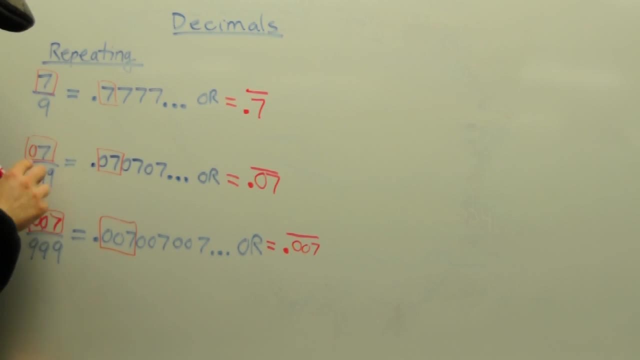 to be. Well, make sure you have the same amount of digits in the top and the bottom. Okay, So 2,, 2,, 3,, 3, and then you say, okay, well, the repeating part is simply going to be the. 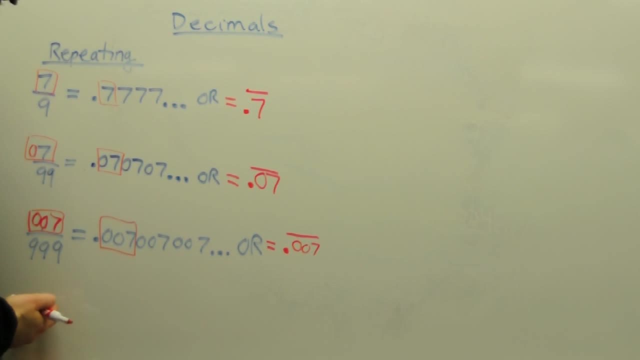 top two digits. That's the case when you have 9,, 99, or 999, or continuing the pattern 9, 9,, 9, 9, stuff like that. That's one thing. It's a very important pattern and in the next little video I'll show you an alternate. 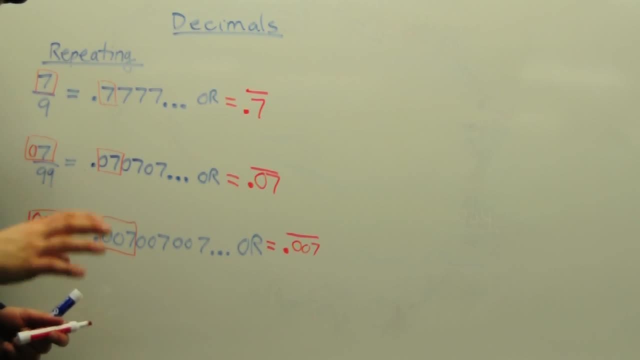 pattern. that looks very much the same, but it's not, So I'll do that in the next video.